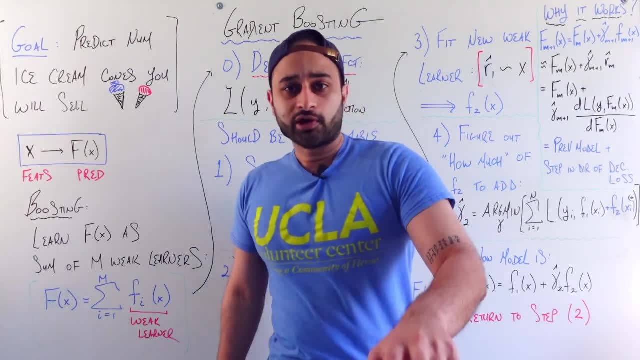 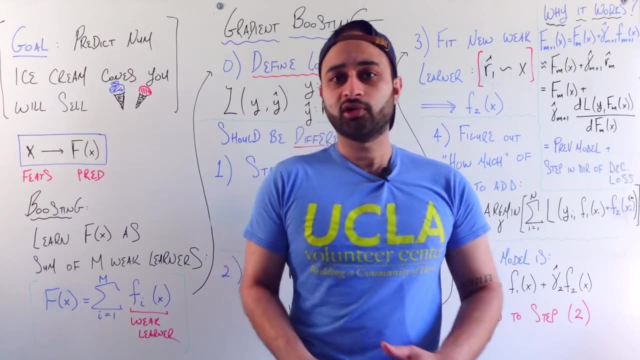 a lot stronger of a statistician or a data scientist, And so let's go ahead and get started. We're going to start with a real-world situation, as we always do. Let's say you have the good fortune of owning an ice cream shop and you're trying to build a model which is going to predict. 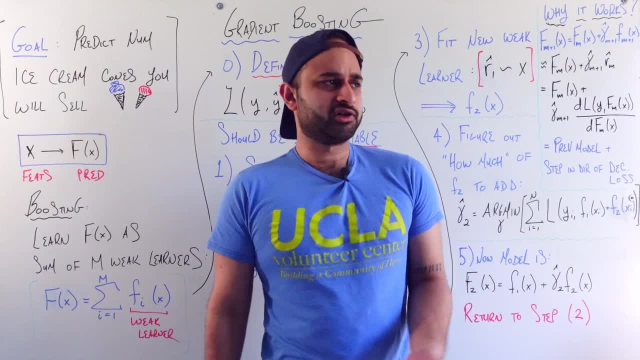 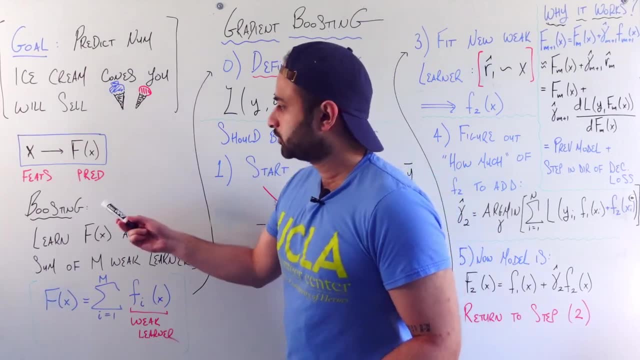 the number of ice cream cones you're going to sell on any given day and that there's some features out there. Let's say you're going to use temperature the day of the week. there's some list of features you can use in your model And so in a little picture you're trying to take those. 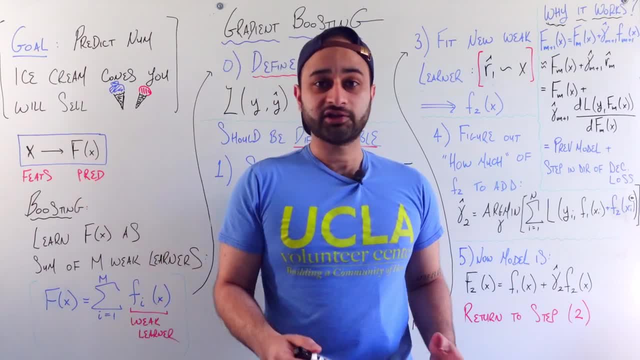 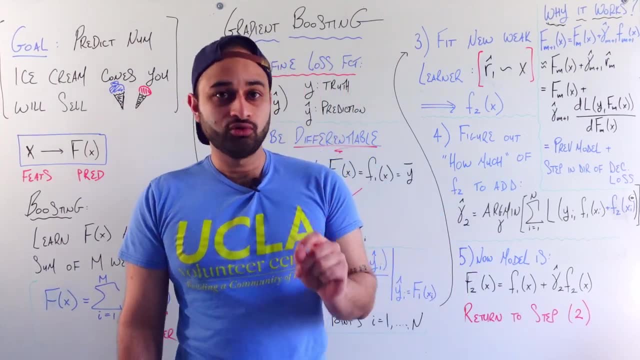 features x and learn some kind of prediction function f, which is hopefully going to tell you how many ice cream cones you sell on any given day. Let me pause here and talk about the first pro of gradient boosting, which is that, although we're clearly trying to solve a regression problem, 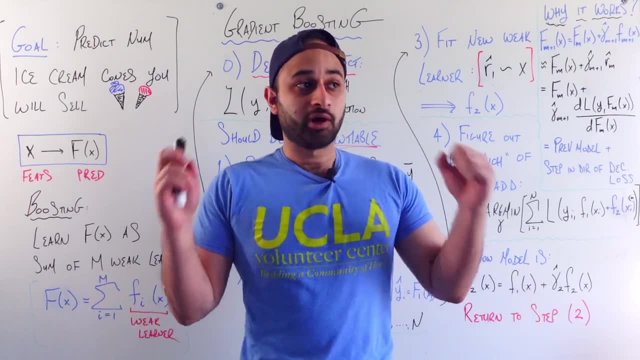 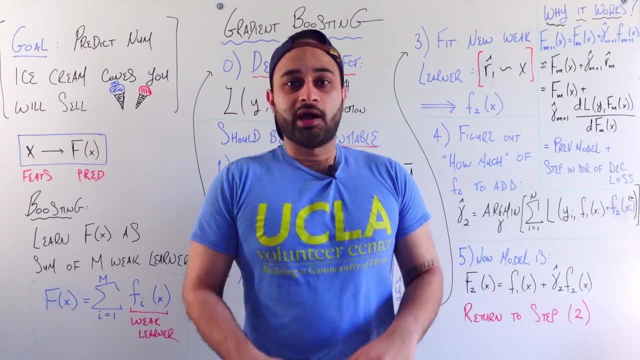 today. it's some kind of continuous variable we're trying to predict. gradient boosting can solve, yes, regression problems, also classification problems, also more exotic things like ranking problems and other things as well. So it's this kind of general purpose framework that is not just. 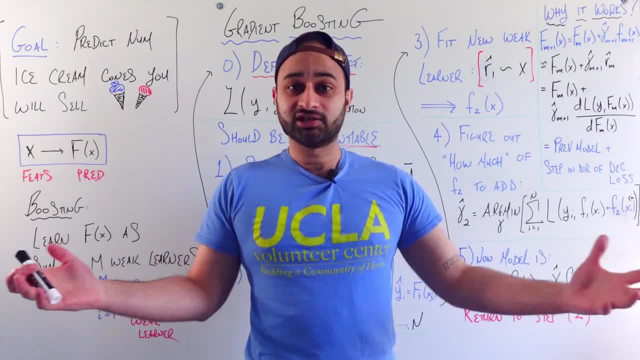 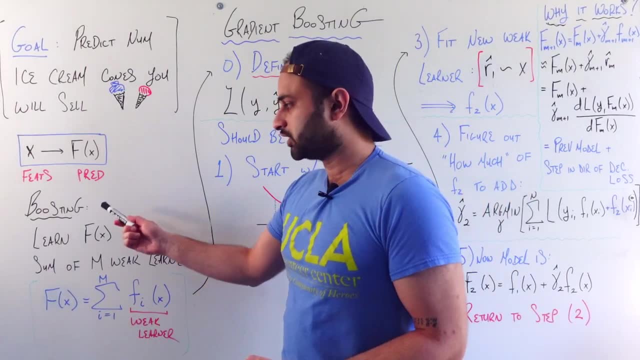 good for one type of problem. It can really solve many, many types of problems. So that's one of the big flexibilities it has going for it. And now let's talk about the first word in gradient, boosting, which is boosting. If you haven't learned about boosting before, it can be somewhat of an interesting, weird concept. 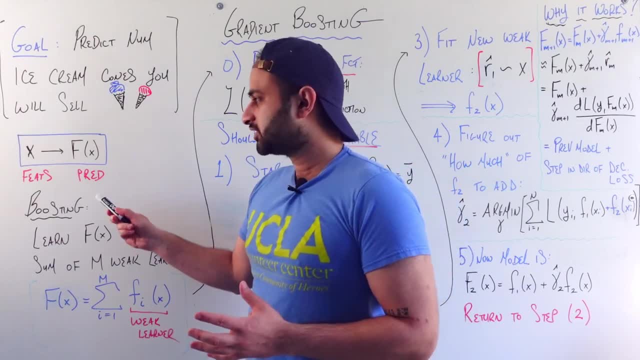 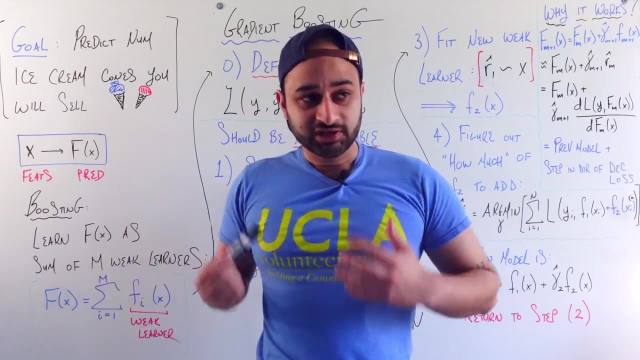 So let me try to break it down before moving forward. Boosting says that when we learn this f, so we're going to have some kind of final prediction function f model. at the end of the day, we're saying that boosting is saying that we're going to learn f as the sum of m- weak learners. 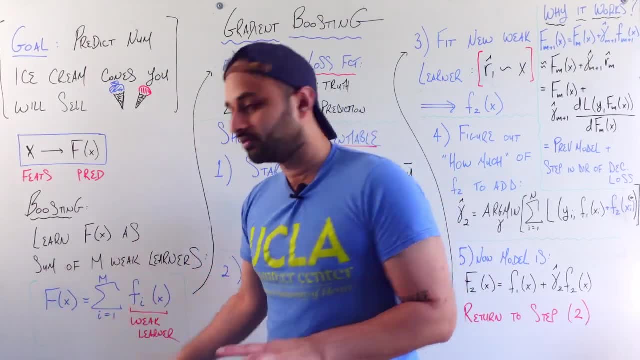 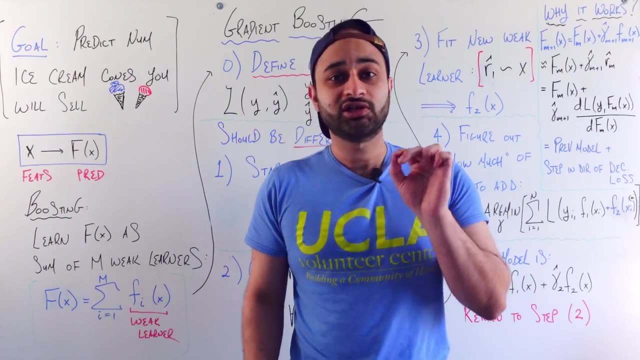 So mathematically it looks like this: Whatever function we learn at the end of the day is going to be able to be expressed as: the sum of i equals 1 to m of these f, each of which is what we call a weak learner. 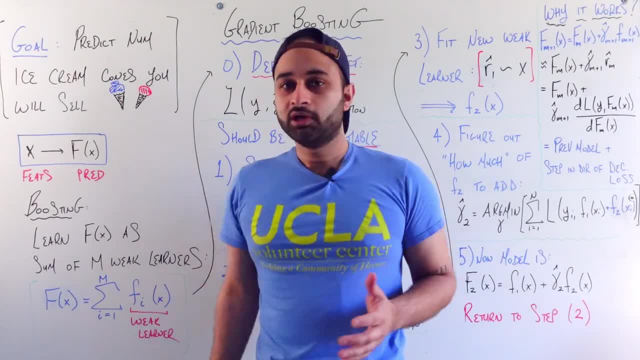 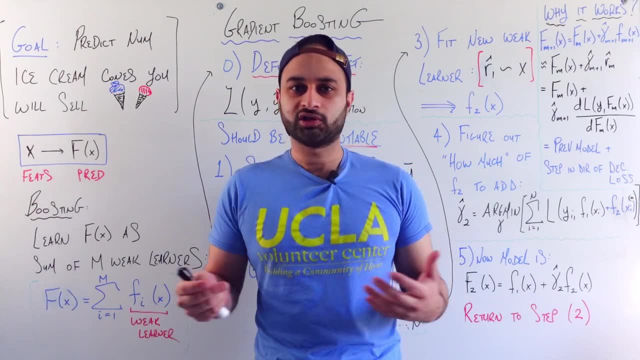 Now a weak learner, for example. this is a regression problem. You can think of a weak learners, for example, a underpowered linear regression or underpowered support vector regression or any kind of regression model you've learned so far. The only condition is that it should be underpowered. 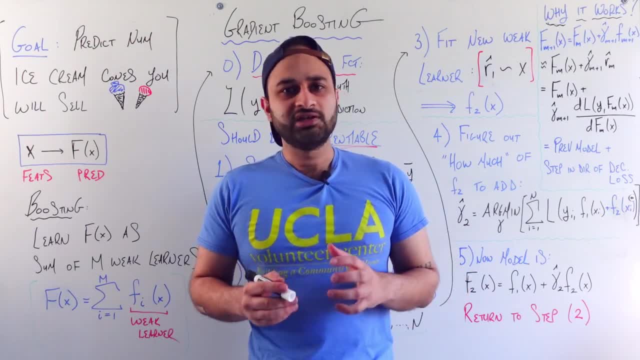 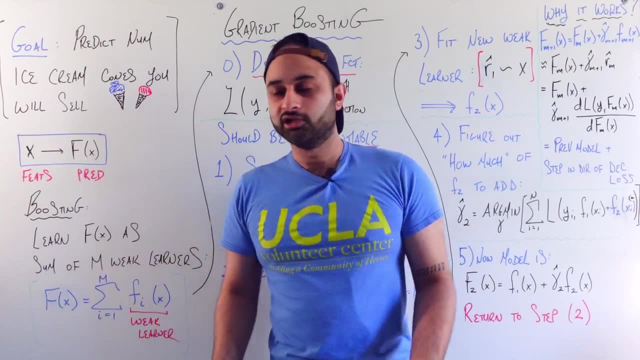 It should not be too complicated, And this phrase is kind of more of an art than a science, but basically means that you're not trying to kind of capture all the dynamics in your data in just one of these weak learners. You're trying to capture some of them, but the idea of boosting is that the next weak learner that you train 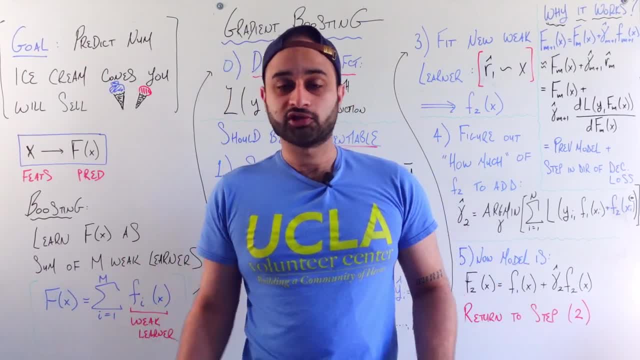 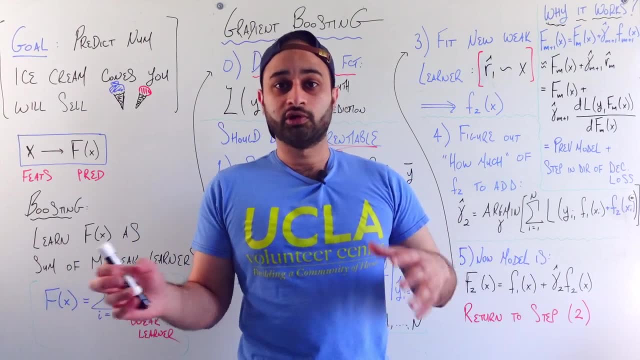 is going to learn from the mistakes of all the weak learners that came before it. So you train some really bad weak learner first, The next one learns from the mistakes of that one, The one after that learns from the mistakes of the first two, and so on and so on. 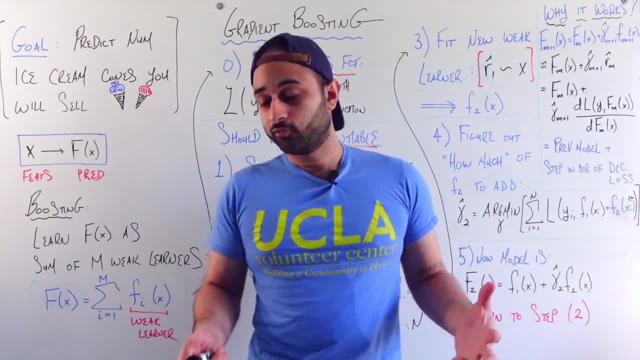 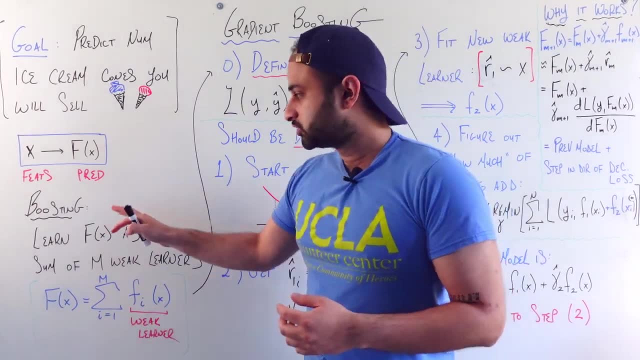 So that, at the end of the day, although each of them is weak by itself, when you combine them together, you end up with something that's actually extremely powerful. OK, so that is the idea of boosting. Now let's go into the step by step process of gradient boosting. 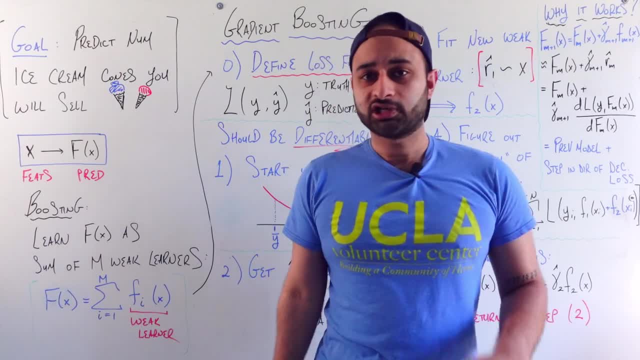 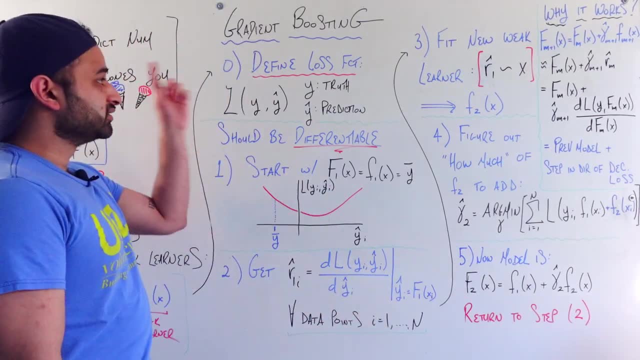 and I'll make sure to explain the intuition and the interpretation along the way. So let's start with step zero. It's called step zero because it's not really part of the process, but it is crucial, something you have to decide on before starting, which is define your loss function. 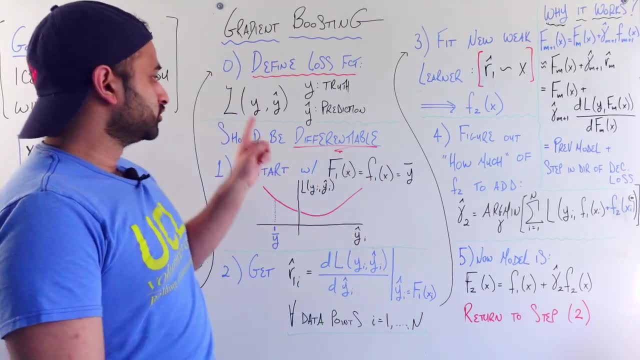 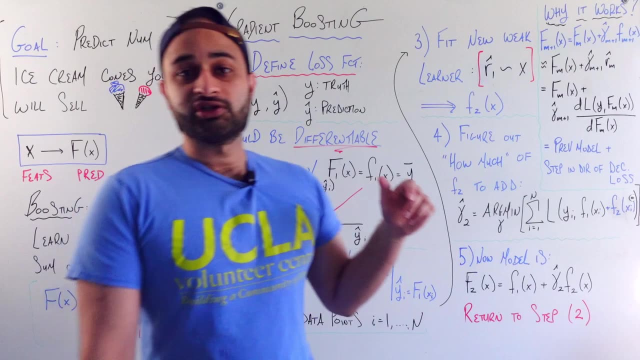 So you need to decide some kind of loss function which inputs two things: The true label, in this case, the true number of ice cream cones you sell on any given day, and the other thing being the prediction y hat, which is the. 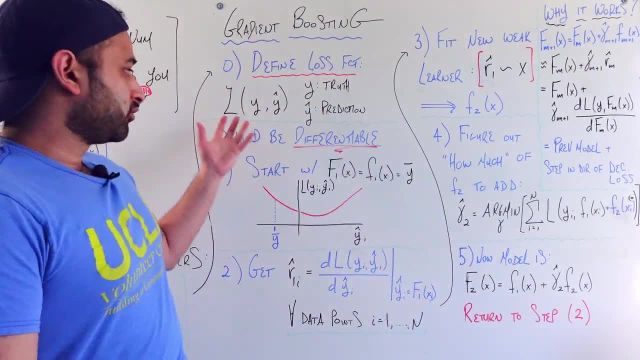 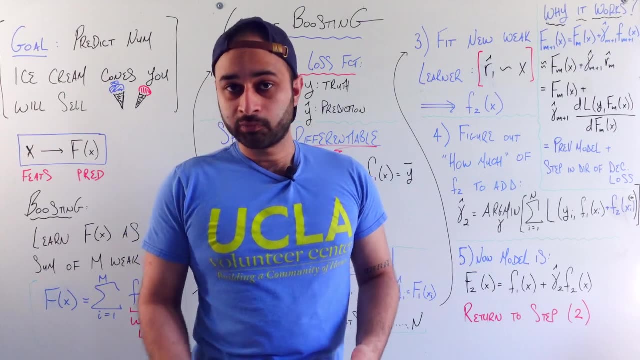 output of your gradient boosted model so far. And, of course, the higher the loss function is the worse job you're doing, the higher loss you have and the lower the loss function is the better job you're doing. Now this loss function needs to satisfy one other condition which is very important. 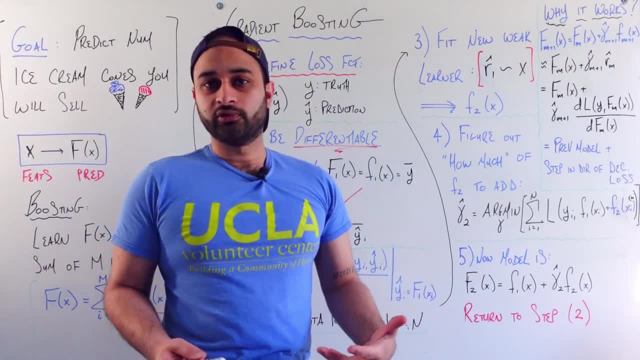 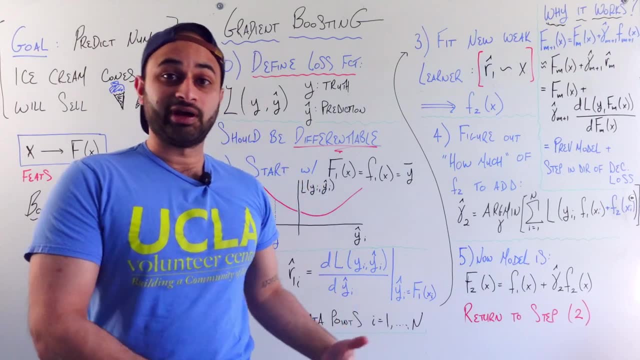 which is that it needs to be differentiable, and hopefully differentiable in some kind of efficient, quick way. This goes hand in hand with the fact this is called gradient boosting. If we can't easily take gradients of our loss function, this is not as easy as if we can. 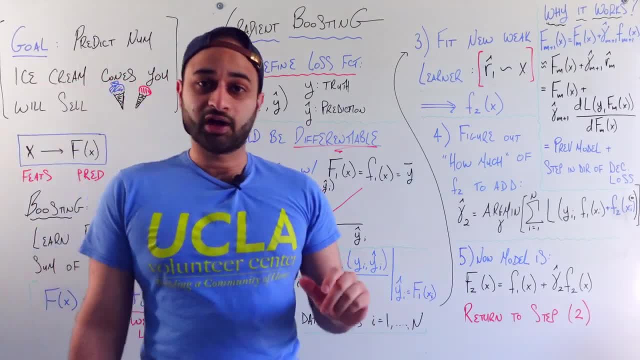 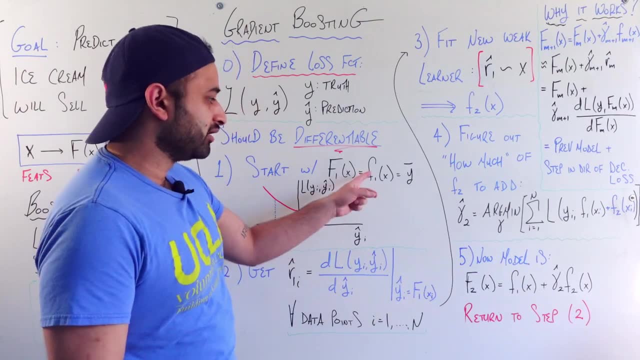 So we need to pick some kind of differentiable loss function here and now. we can start with the process Step one. Step one of the process is that we're going to start with some extremely weak learner f1 of x And, for example, we can just take the mean of all of the number of ice cream cones we've sold in our training data. 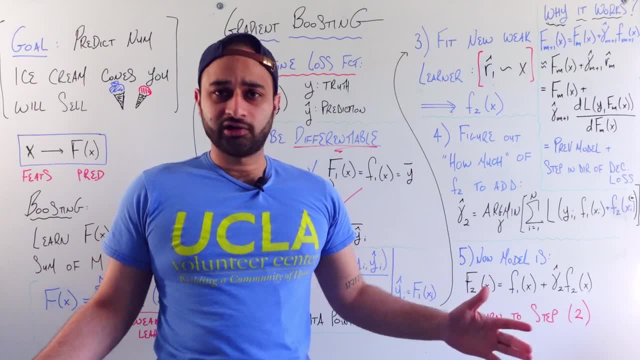 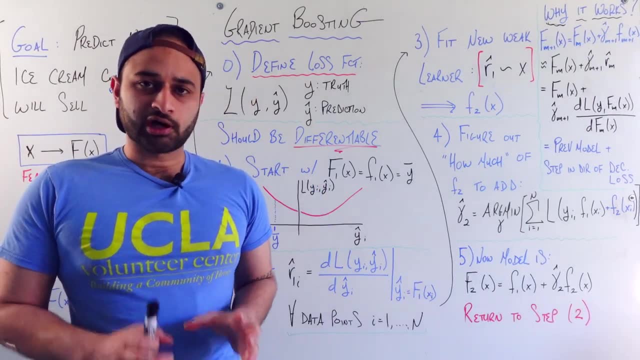 and that can just be our first model. Clearly a terrible idea, clearly a bad idea to just predict the mean for every single day, but it's starting somewhere. And now to kind of throw a picture in here, if we plot the loss function, so, for example, if you pick one option, 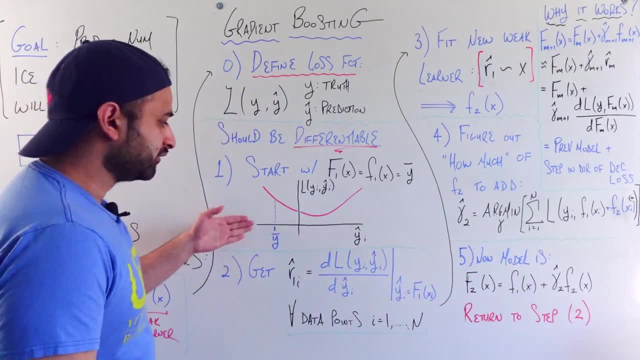 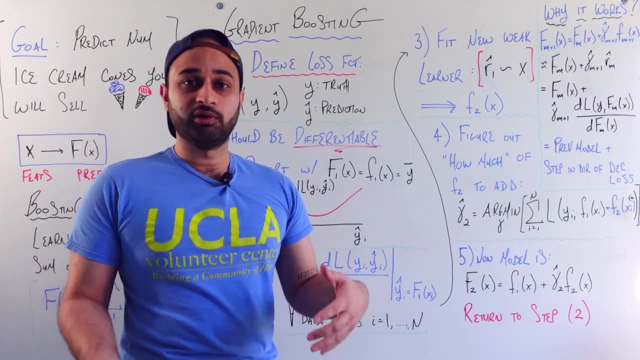 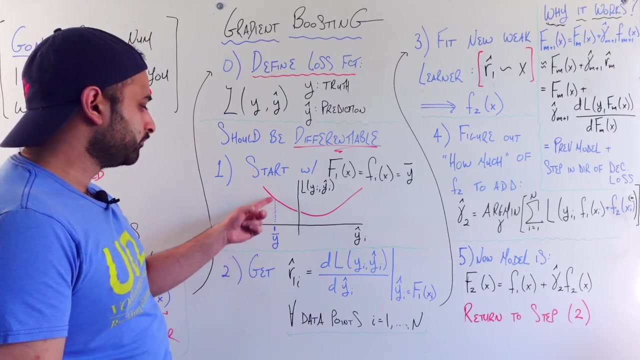 observation in your training data i we can make a plot of the predicted value of this guy against the loss function, which is the true value and predicted value being put in there, and give us the loss function on the y-axis. And, for example, let's say that the current prediction we have, which is the average of all the y's, is here: 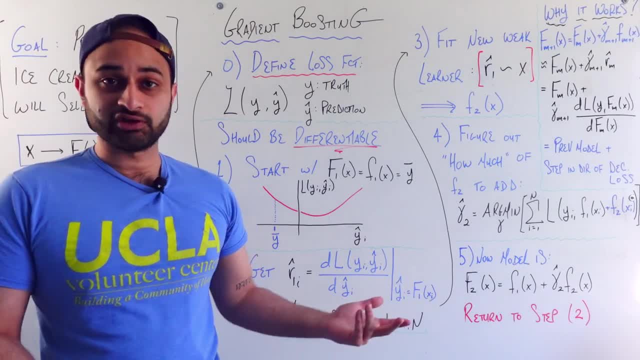 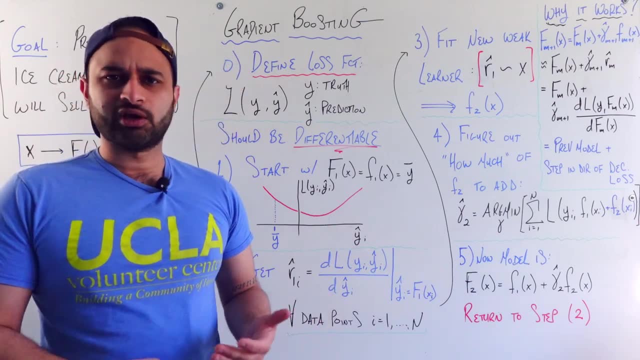 So clearly we're not doing as good of a job as we could for this observation. There's clearly many other values of this predicted value that could give us a lower loss, And so that's kind of just saying we're not done yet. But this picture is going to help us kind of understand what comes next. 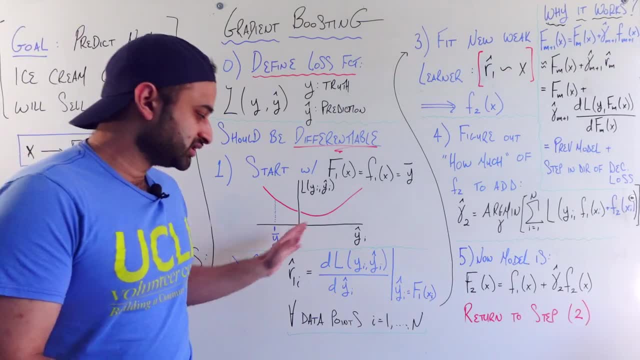 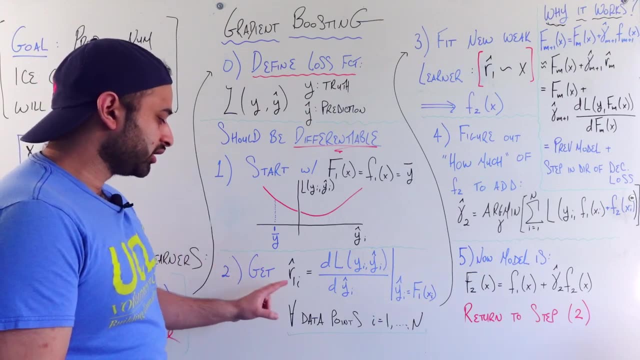 Speaking of what comes next, the next thing we do- and this is the key step. OK, step two is the key step, so it's going to be helpful to understand. I'll spend some time on it. We are going to compute these quantities. 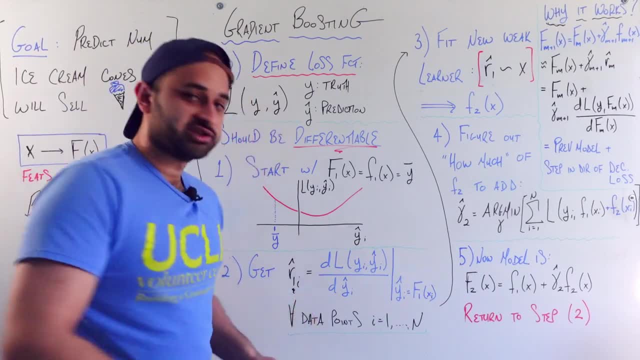 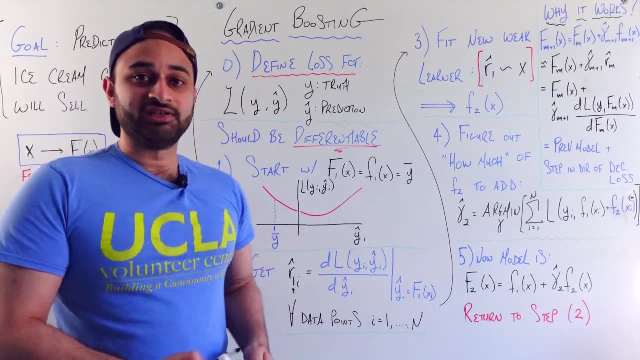 R1i. this one is basically just saying that we're currently looking at the first weak learner. This one is going to get updated as we move on. This i is just the data point we're currently interested in, So i is going to go from 1 to n if we have n data points. 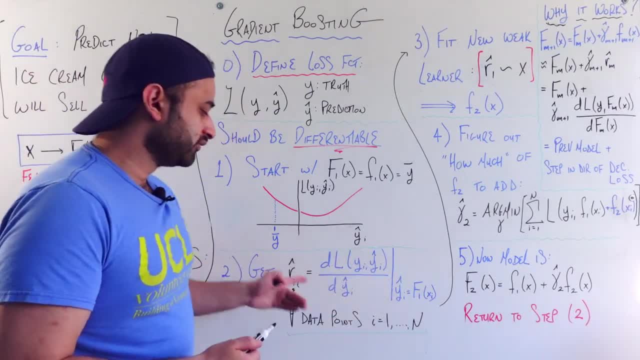 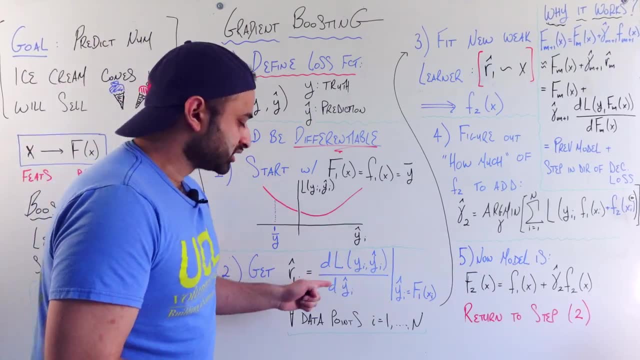 So for each data point, we're going to compute this derivative or this gradient. This gradient is the derivative of the loss function, which is this guy with respect to the prediction that we currently have right now, And that's what this guy is saying here. 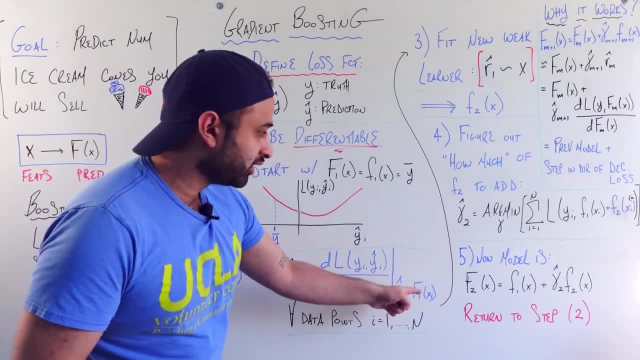 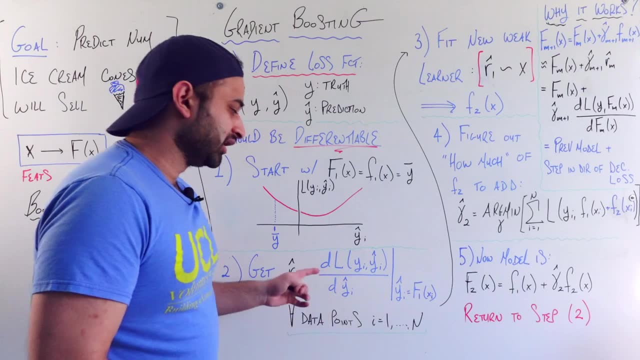 We're saying that if we plug in the current prediction, which is F1, which is exactly what you see here, which is currently the mean of all the y's, then this is going to give us the gradient Now very mathematical, so far. 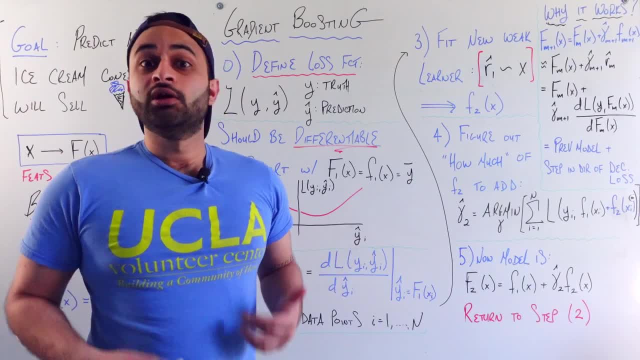 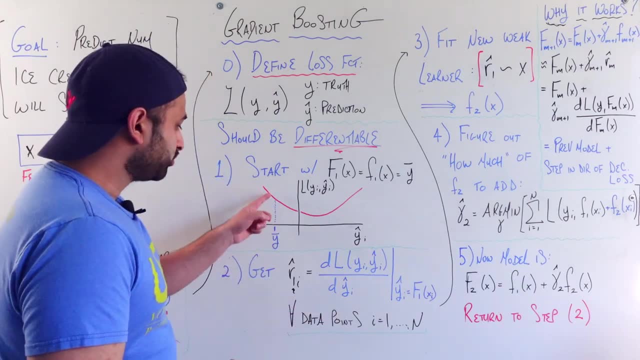 Let's look back at this picture to make sure we understand what this means graphically. If I take the gradient of the loss function for this current observation, i at the place that the current prediction is, then I'm basically getting this gradient right here. 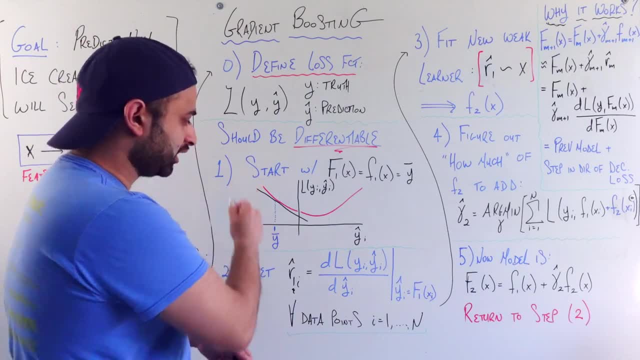 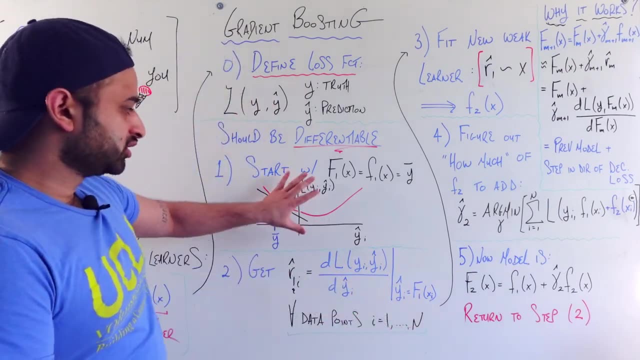 That's more curvy than I would have liked, but that's supposed to be a straight line gradient right there. And another key thing is that we do the exact same thing for all data points. i equals 1 to big N, So this is just the picture for one possible data point. 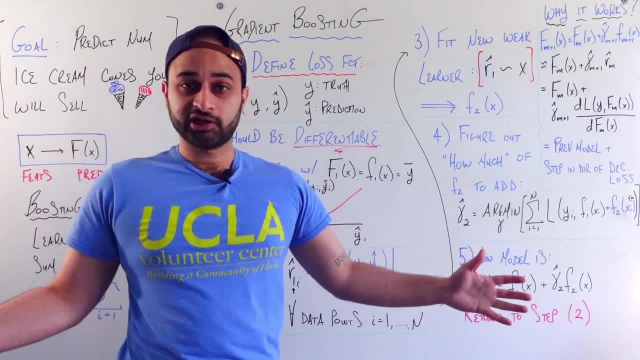 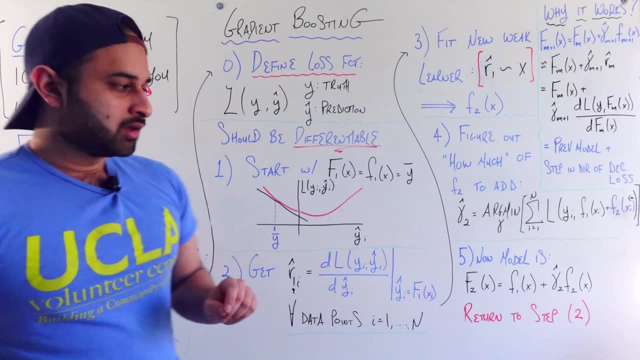 We have similar pictures of loss functions for all of our data points and we compute all N of these gradients and those get stored in these r variables. Now why did we just do this? We did this because we would like the next weak learner that we learn. 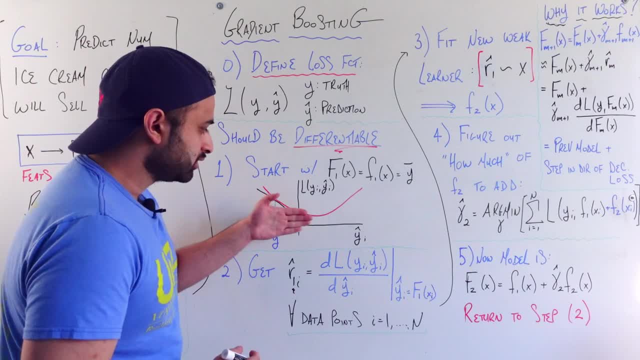 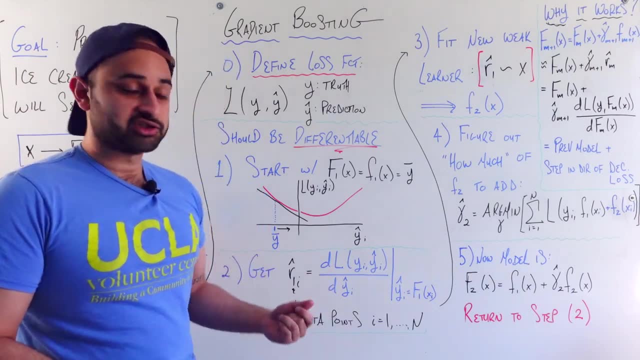 to hopefully move this prediction in the direction of the decreasing loss. So, for example, if I move this a little bit this way- and I know to move it that way because the gradient I just computed is negative- if my prediction was over here, the gradient would have been positive. 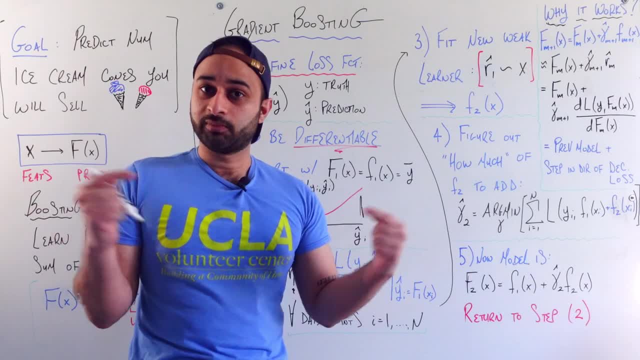 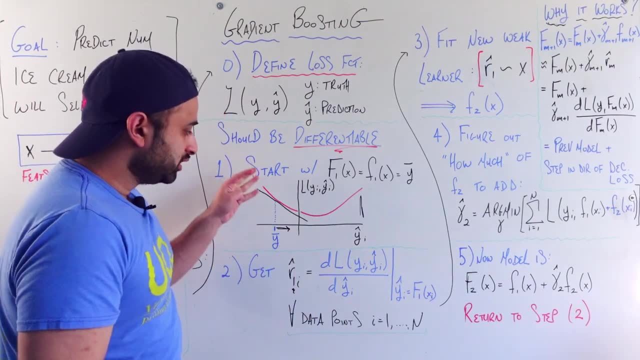 and I know to move in the other direction. So the gradient is informing which way am I supposed to go to minimize the loss on each of these different examples. So if I take a little step in this direction, then I'm going to be on my way to decreasing the loss on this particular example. 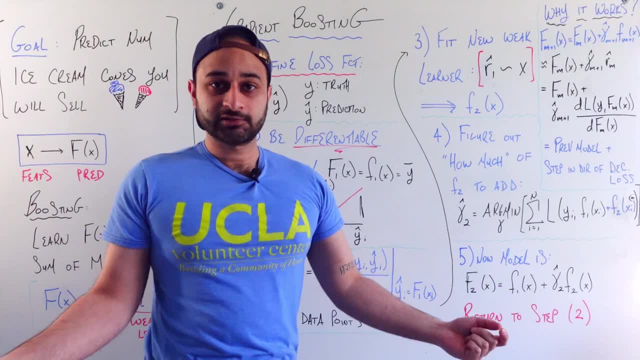 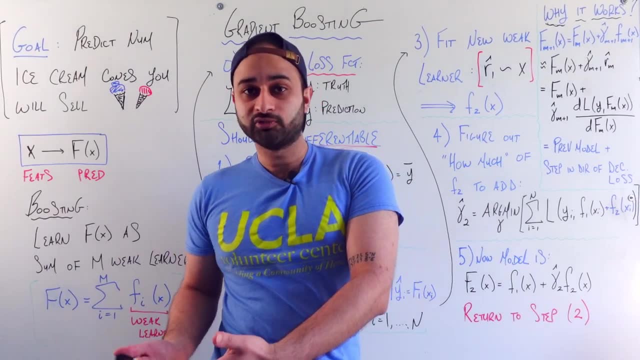 and also every example, if I kind of generalize this process. So that's the idea. So now step 3 is that we fit that next weak learner. So here's where that next weak learner comes in: learning from the mistakes of the old weak learner. 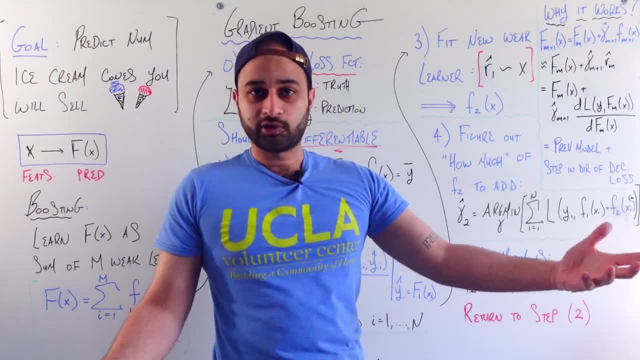 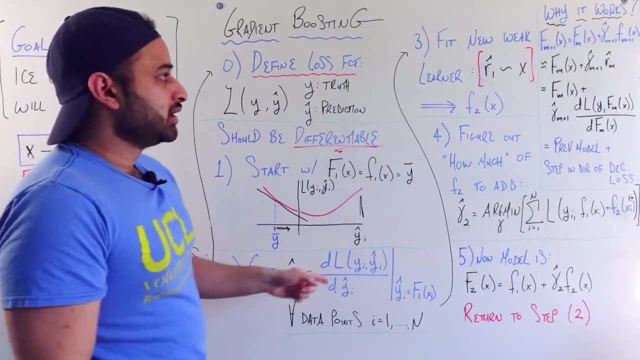 So the way we fit this new weak learner is we learn some kind of model, a weak model, where the target variable is r1, hat. which are all these gradients? and the inputs are the same features we've always been using. So the one thing that stays constant in this entire process: 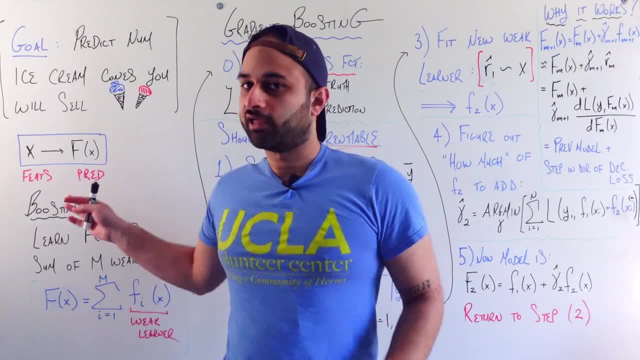 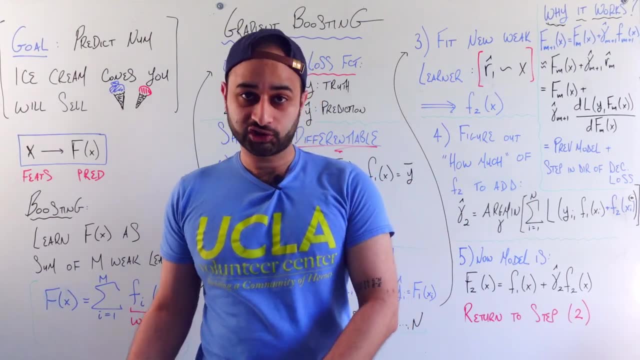 is that each weak learner is trained on the original set of features we were looking at the whole time. And, for example, let's say our weak learner is a linear regression, then this f2 of x is going to be that weak learner linear regression. 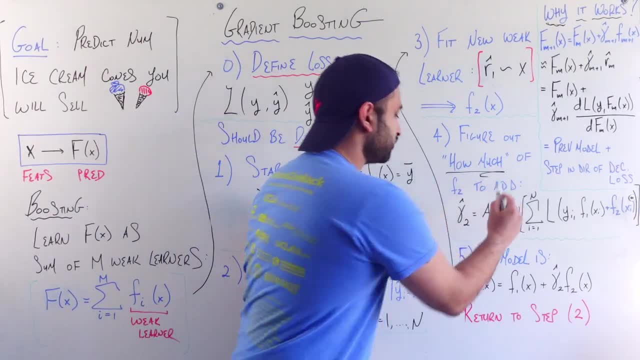 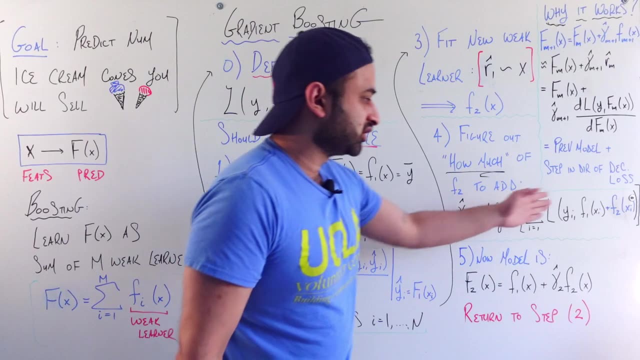 And now what we do is figure out how much in quotation marks, how much of f2 to add to the current model, which is just f1 of x, And we do that by solving this problem. It looks complex, but let's just kind of break it down. what's going on? 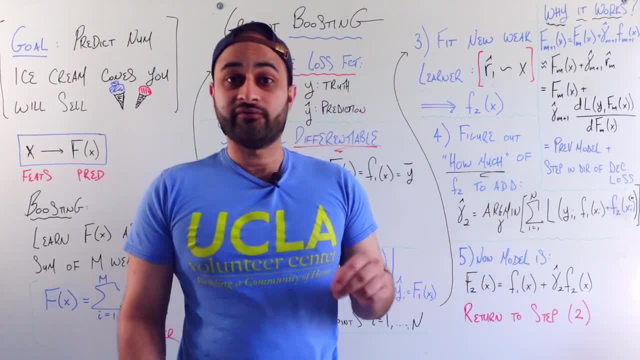 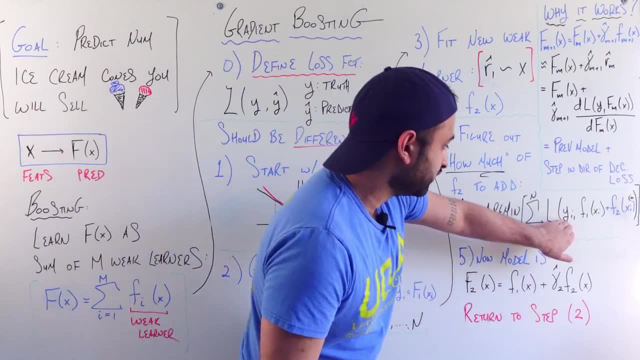 This inner part is summing over. i equals 1 to n, which is every single data point. We're just summing the loss for every single data point, The loss from putting in the true value yi and putting in the proposed new prediction. 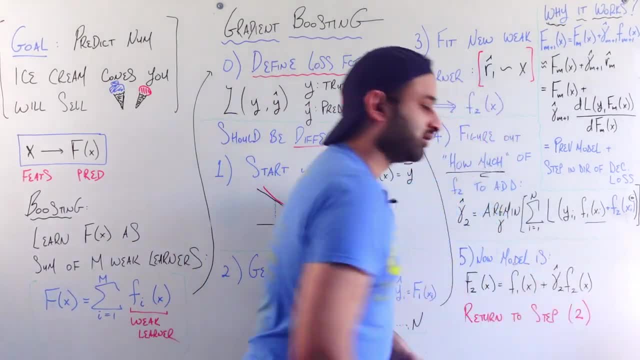 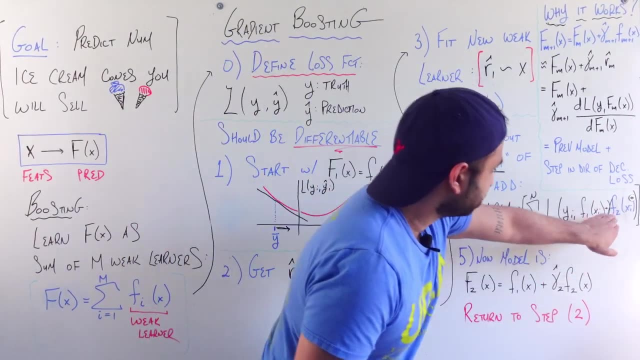 which is going to be the old model f1 of xi, the old weak learner. plus I just snuck a little variable in there, you probably noticed, but plus gamma. so that thin thing, right there is the same variable gamma you're seeing here. 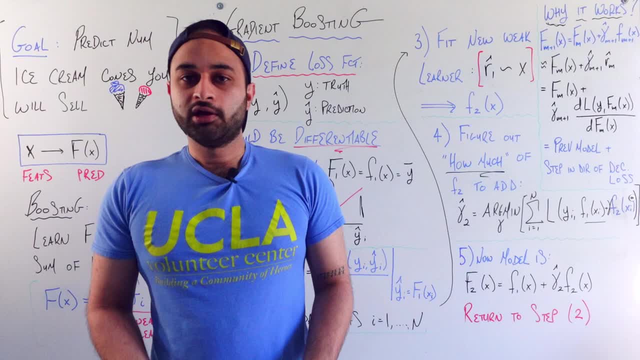 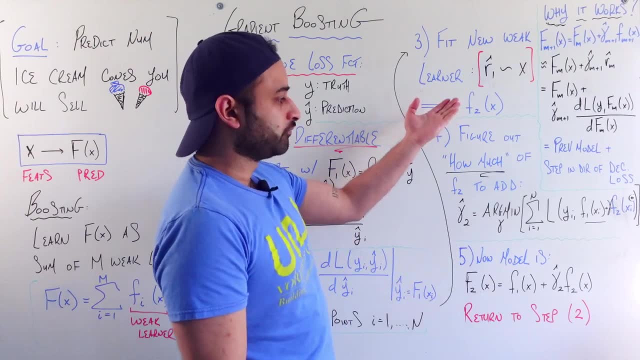 plus gamma times the new weak learner. So you can think of this as just some kind of recipe. It's saying that I know that I'm going to add some quantity of this new weak learner to my model. so far, This is just saying: how much do I want to add? 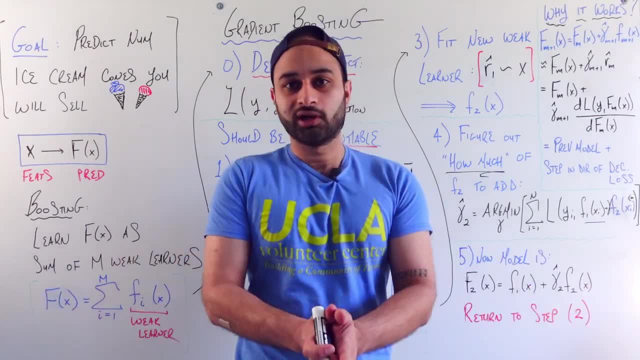 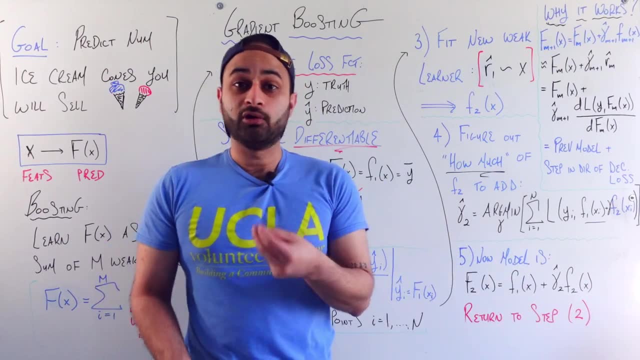 because I don't want to add too much, I'm going to overshoot. I don't want to add too little, I'm going to undershoot. So this is officially called a line search which looks for the correct gamma, the correct amount of the new weak learner to add. 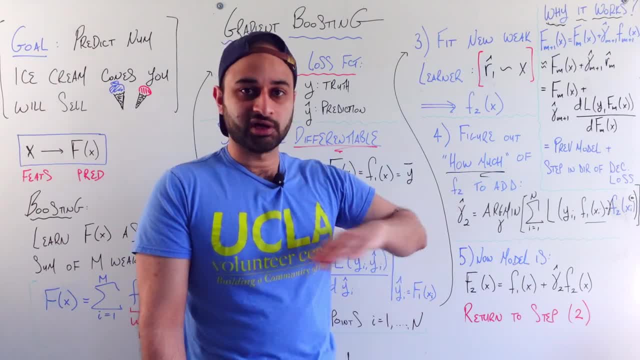 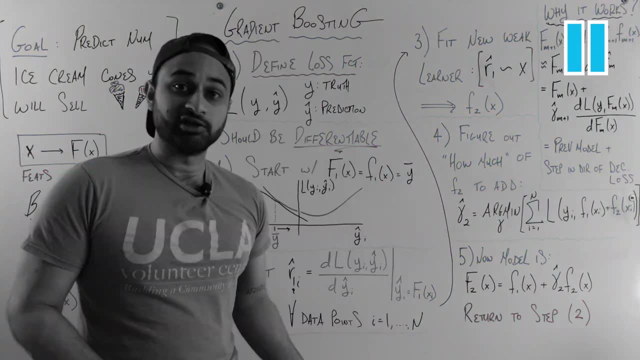 to the existing model so far, which is going to minimize the sum across all loss functions for all n observations, and the answer to that is going to be gamma to hat. Hey, sorry to interrupt you. passwordpick, Just realized while editing this video. 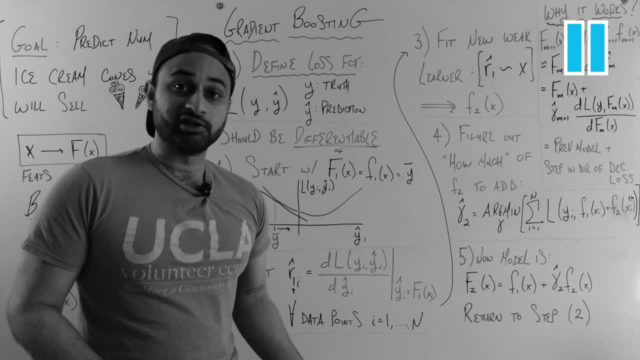 all of the math is correct here. It might have been a better idea to put a negative sign in front of the gradient to make it match more like gradient descent, and that way our gammas are always going to be positive, the amount in which we travel in that direction. 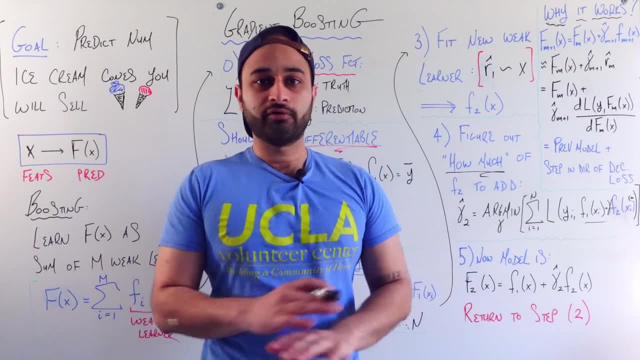 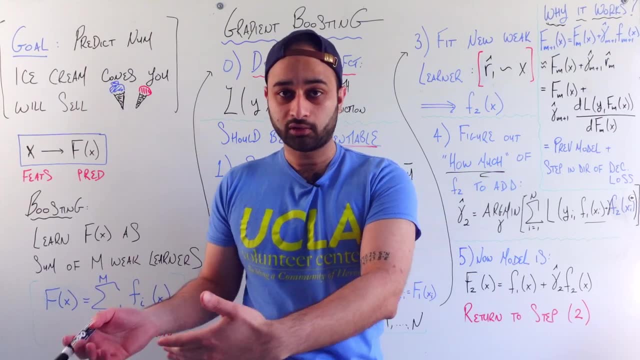 And that's it. We've done one iteration, we've worked through all the math, all the intuition we need and now we can officially say that the new model. so we've only done one step so far, but now our model is big F2 of X. 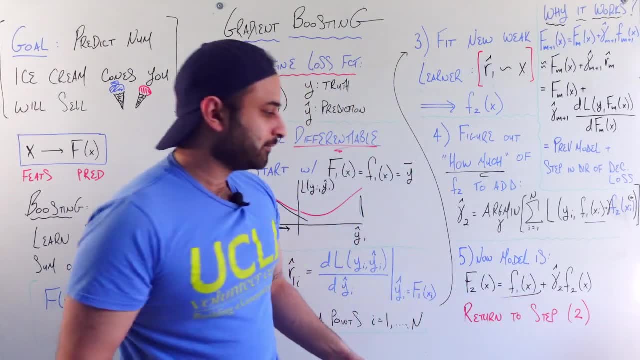 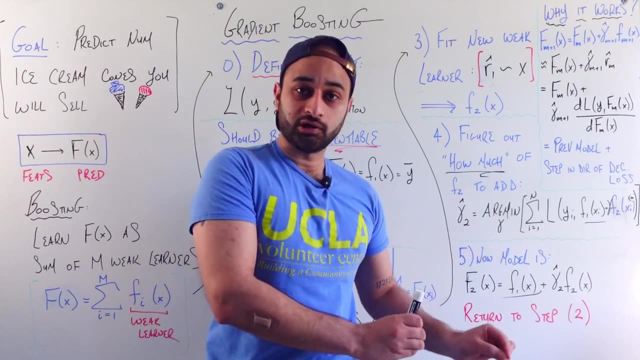 which is equal to the old weak learner, which is this guy plus that amount of the new weak learner, And this is going to do better. this is going to do better than the old weak learner alone, because we have hopefully moved all of these predictions for all n observations. 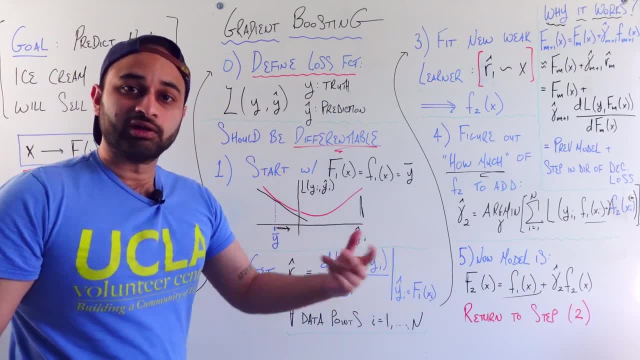 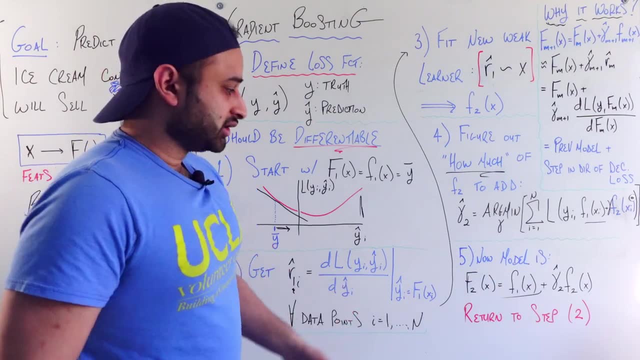 in the direction for which their loss functions are a little bit lower than they were before. So we're getting a better performance, But we're probably not done yet, because this was still just a weak learner, And so the last step, which is just return to step two, 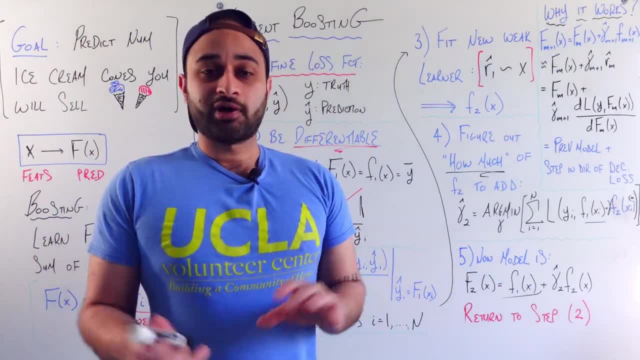 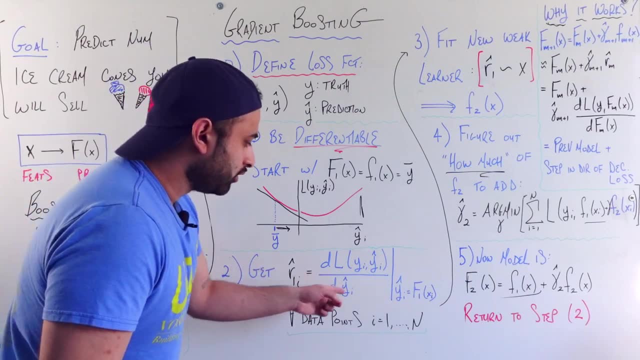 and do this process all over again. So let's talk through the high level steps, just so make sure you understand. So next thing we're going to do is basically get these gradients again. but now our prediction is going to be this: the sum of two weak learners. 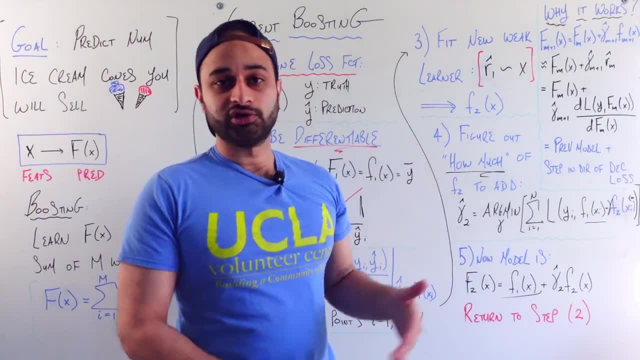 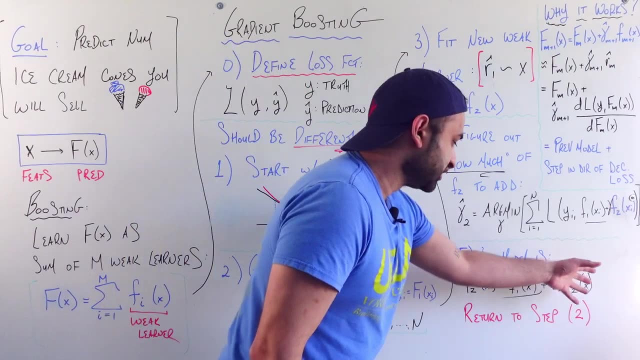 We're going to go ahead and fit a third weak learner on those gradients. using our features. We're going to figure out how much of that weak learner to add to the existing model And then we're going to say our updated model is equal to this guy. 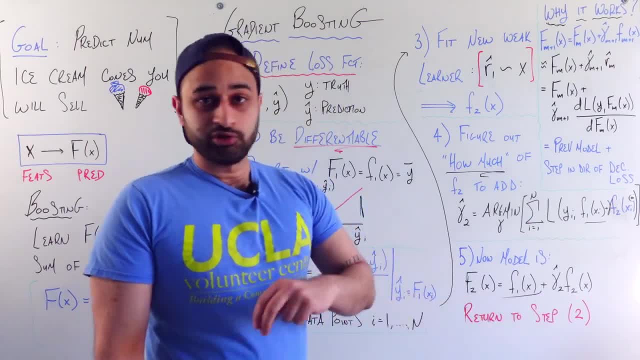 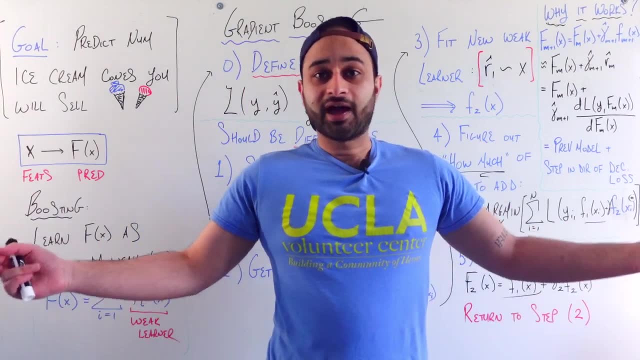 plus gamma, three hat times F3 of X, And we just go on for as many iterations as we want, just adding these weak learners step by step, by step. And, ladies and gentlemen, that is gradient boosting. Now, if you're like me, 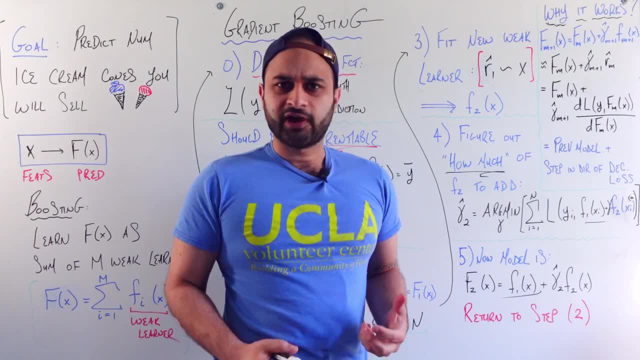 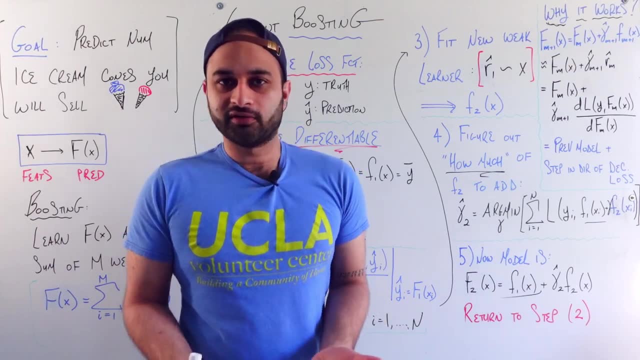 you hopefully understand the process here, but you might not be satisfied with why it works. Seems like everything we did was reasonable, but why does this framework overall actually going to work in the end of the day, And so I think I do owe you that explanation. 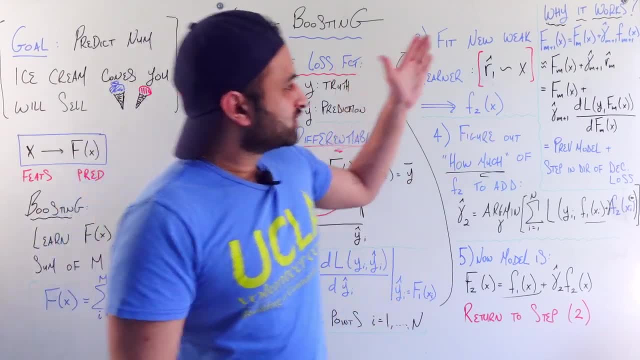 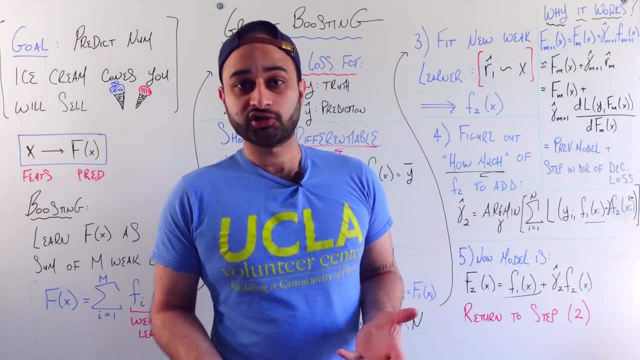 And that's, let's say, the second to last thing we talk about today. So why does this work? Well, think about being at step M, plus one in the process. So you've trained M weak learners so far. So your current model looks like: 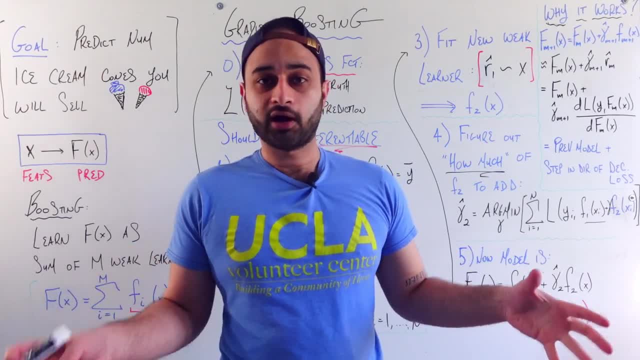 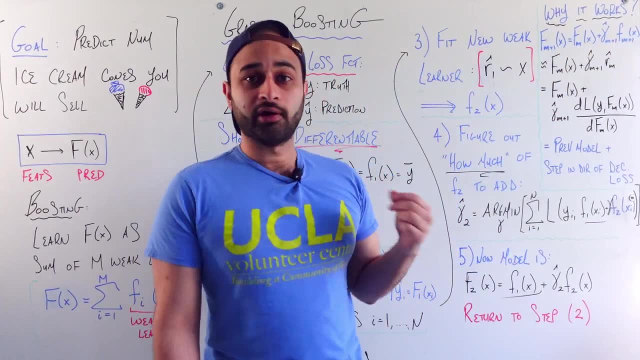 M of X, which is the sum of the M weak learners so far, And now you've proposed some kind of new weak learner. So you're going to add some quantity of this new weak learner- little F? M plus one of X. Why is this doing a better job than F? M of X by itself? 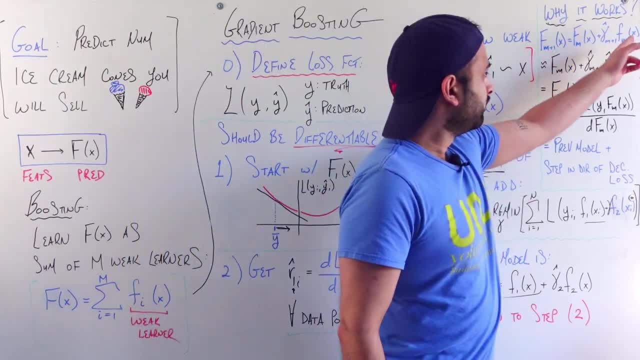 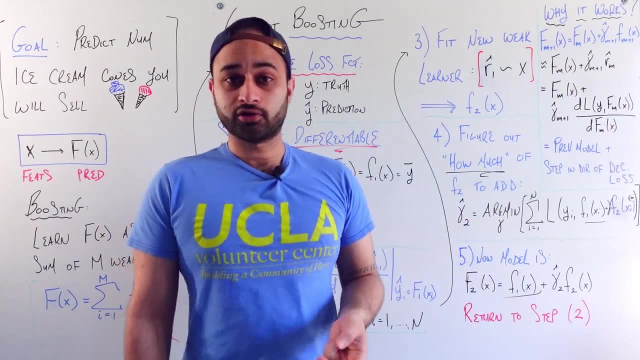 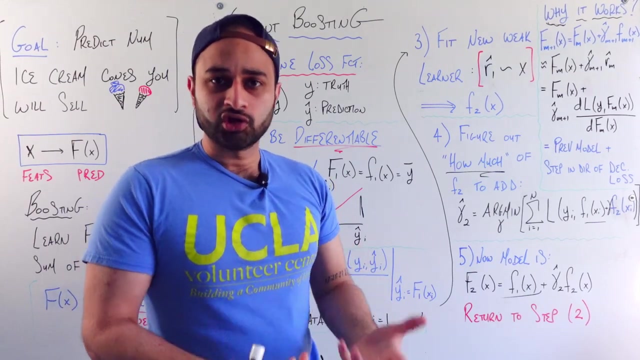 Well, let's trace through everything that we know. This form is approximately equal to the old weak learner, plus this amount plus R hat underscore M. Why? Because this new weak learner plus one X was specifically trained to do a good job. 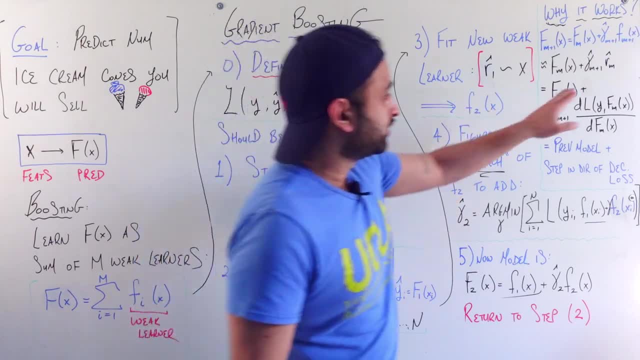 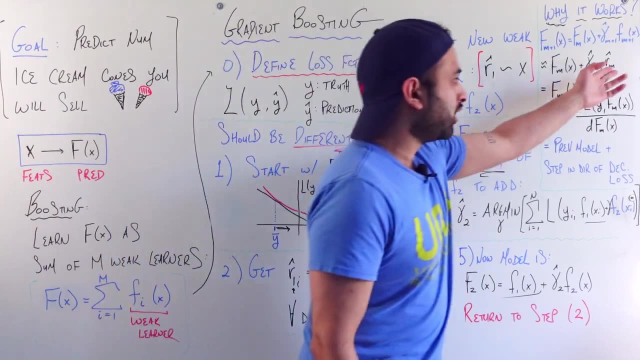 of predicting this R M hat. So we can just put that right there, putting this as an approximately equal to, because it's trying to do as good of a job as possible, being a weak learner. But what is R M hat If we look back at this form here? 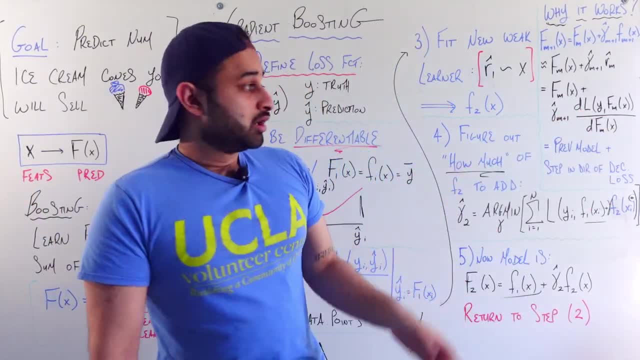 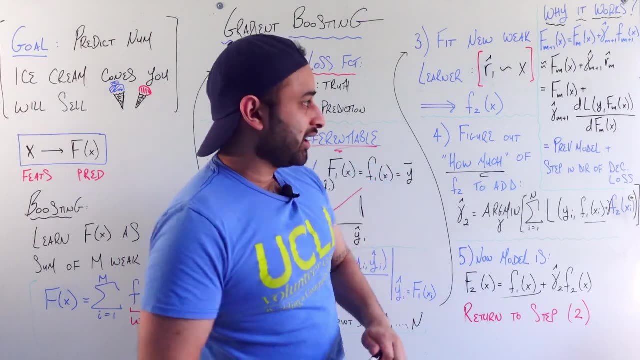 R M. hat is going to be this derivative of the loss function with respect to the current prediction, which is F? M of X. And so, in words, what you're looking at is that the new model, which is F? M plus one of X. 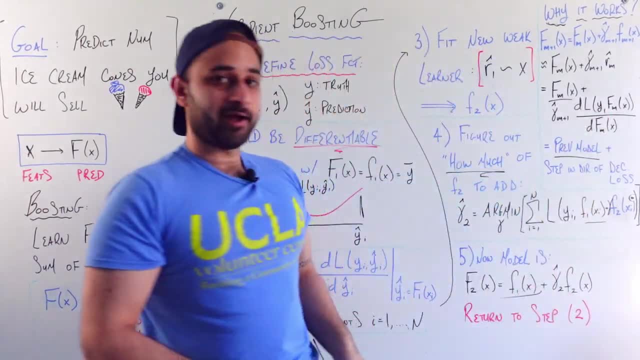 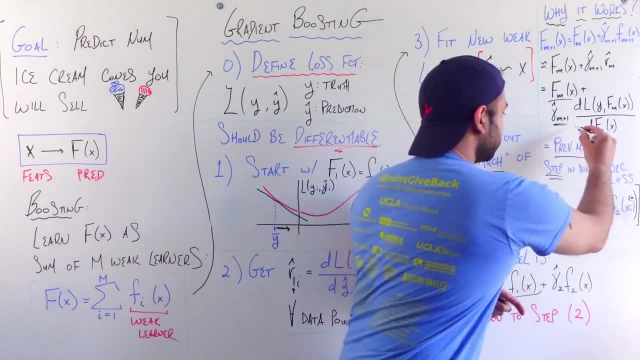 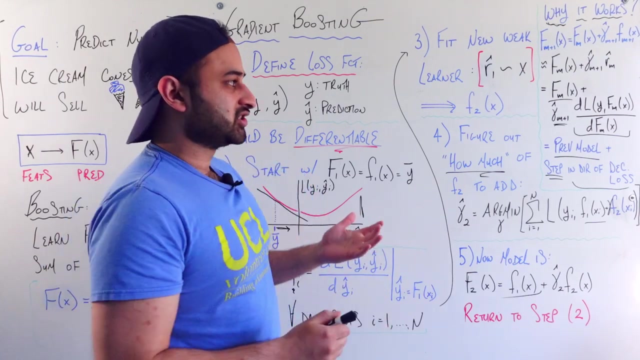 is going to be the previous model, which is that guy plus a small step. which is this small step here in the direction of the decreasing loss, In the direction of the decreasing loss. This is literally just gradient descent folks. This is just saying that we're going to take the previous model. 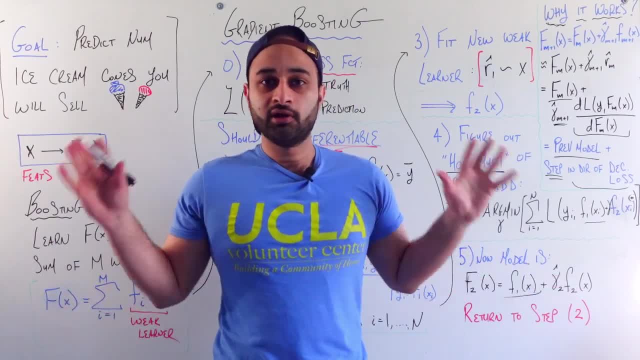 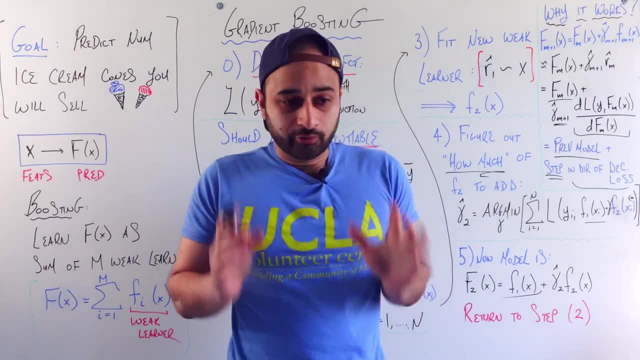 and walk a little bit in the direction where the loss is minimized for all these different data points, And that, hopefully, is an intuitive idea about why this works and why it's so powerful. And now I just want to recap how amazing this is. 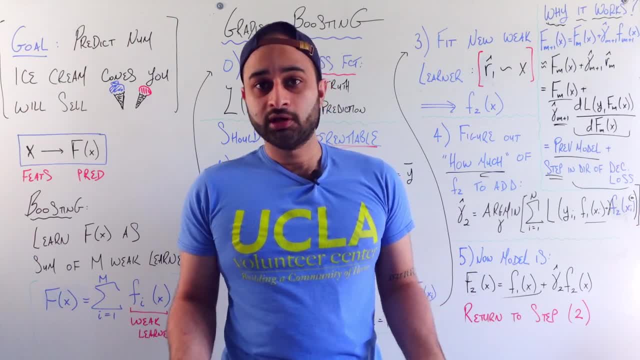 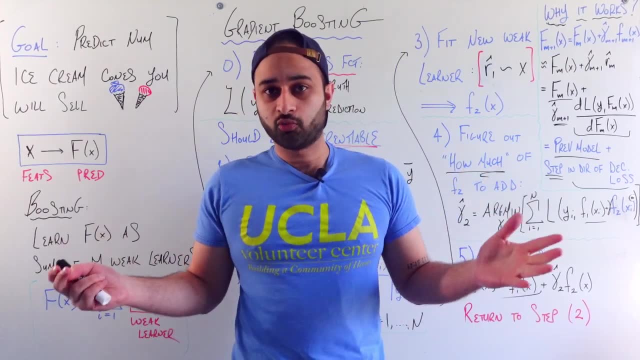 I mean, I know this is a little bit of a longer video than usual, but I think it deserves to be. Look at all the flexibility we have in this process. The problem you can solve: Regression, classification, ranking, whatever else you want. 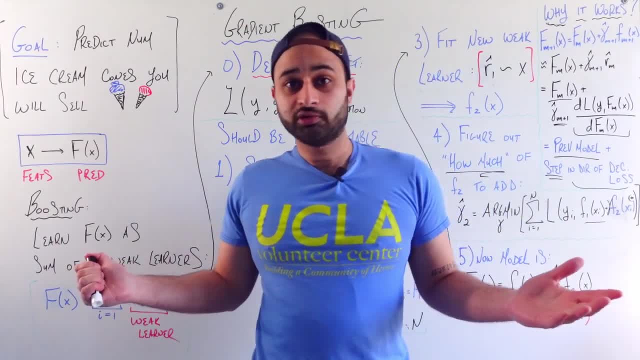 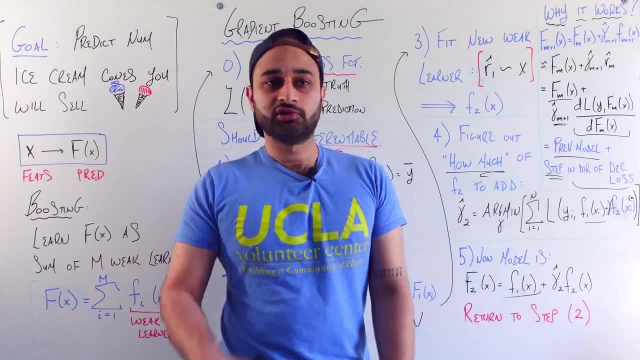 One point of flexibility: The loss function. totally up to you as long as it's easily differentiable. The weak learners that we learn. totally up to you. You're doing a classification problem. Use logistic regression, Use decision trees, Use whatever you want. 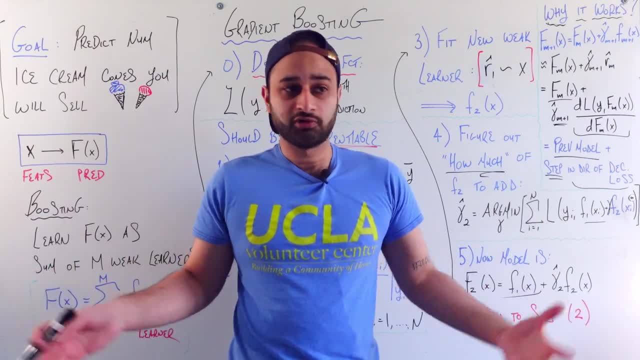 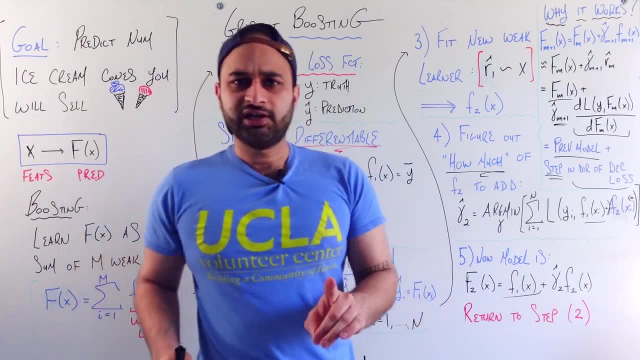 There's so many points of flexibility, such a catch-all framework that does really well in the real world. This is something that you have to add to your tool belt, in my opinion. And now, one note I'll say is that you'll typically hear about the weak learners being decision trees. 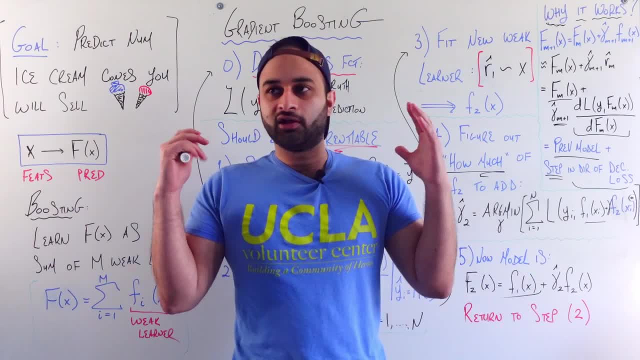 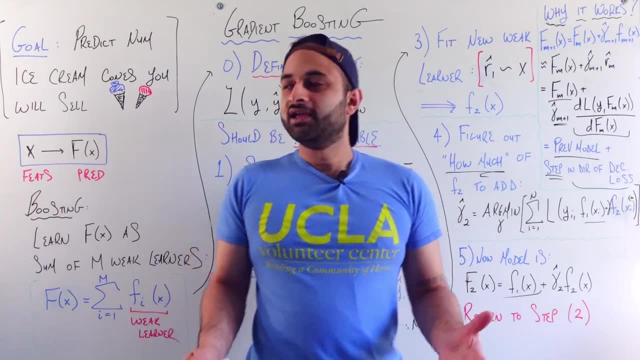 Gradient-boosted decision trees are kind of just a ubiquitous term in the industry and academia now, because we've seen in many, many data sets, many, many different examples that if you're weak learners, our decision trees, whether or not this is a classification. 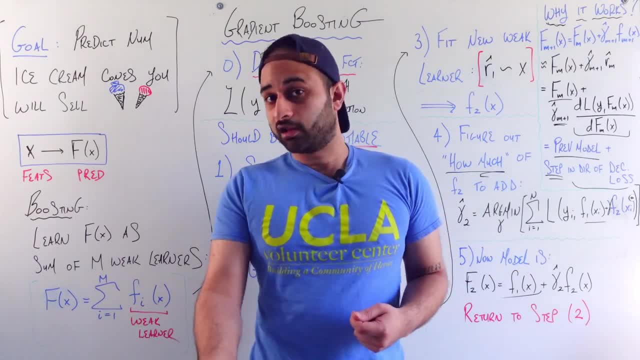 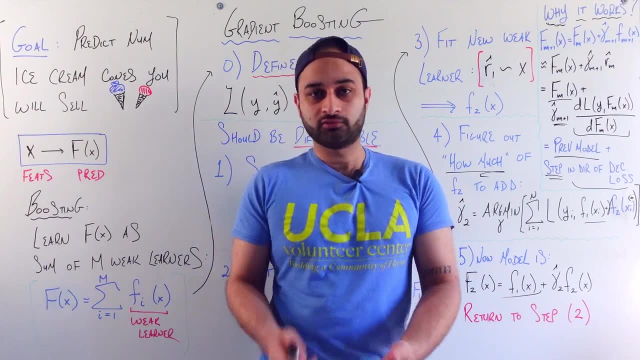 regression, ranking, whatever problem, this does really, really, really well. And now the final thing I'll say, before I let you all go, is: we've talked about all the amazing things, but I have to talk about the drawbacks. We have to talk about both sides. 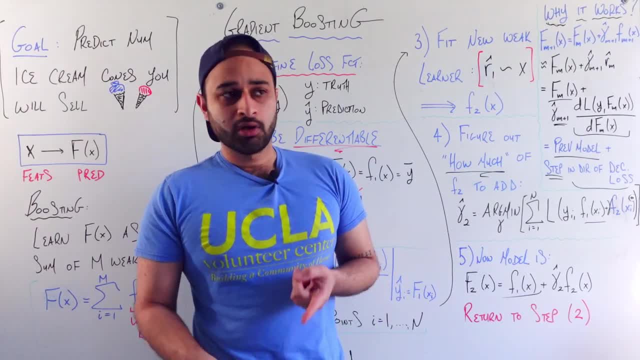 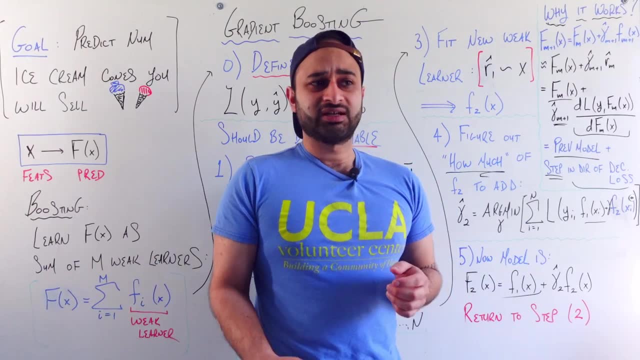 The main two drawbacks here are: first, interpretability: Obviously, we understand, hopefully, how it works, but when you have this model, at the end of the day, which is the sum of all these weak learners, it can be pretty tough to understand or interpret. 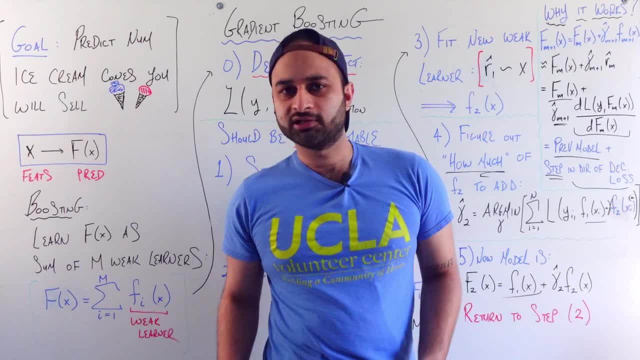 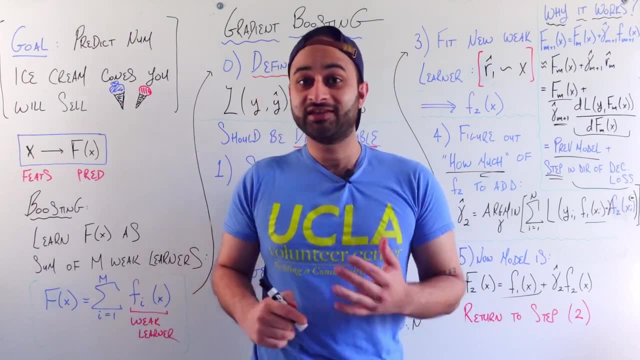 how it actually works at the end of the day. You can use these generic things like partial dependence plots and Shapley values, but by itself, understanding this intuitively is not the easiest thing in the world, So we sacrifice some of that interpretability. 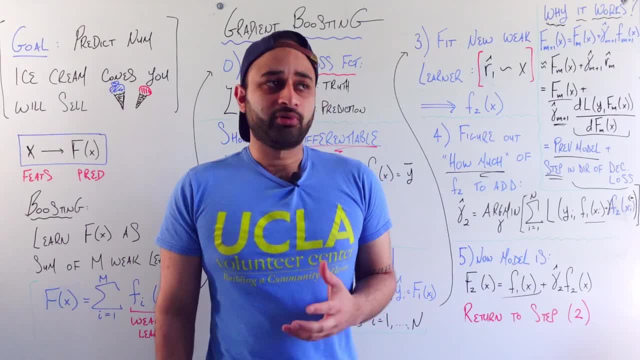 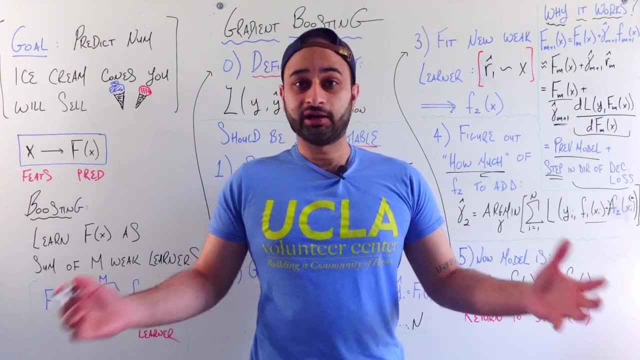 but get a lot of performance gains. The other consideration is that it could be pretty computationally inefficient. There's a lot of moving parts here, so you might need kind of high computing power, especially if you have big data in this situation. Oh yeah, maybe one last thing is that